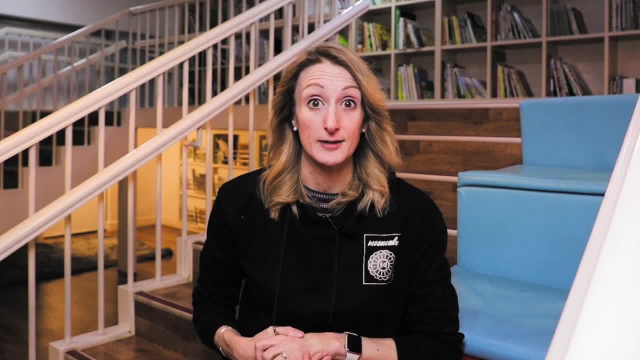 Today I'll be sharing a fun drilling game that will have your students speaking English quickly. So let's get started. So, without further ado, let's get started To play this game. all you're going to need are three sets of flashcards. 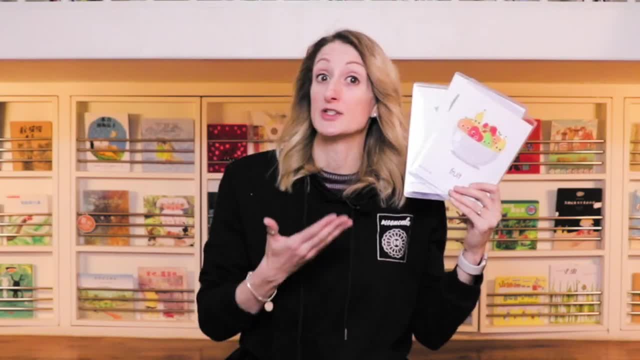 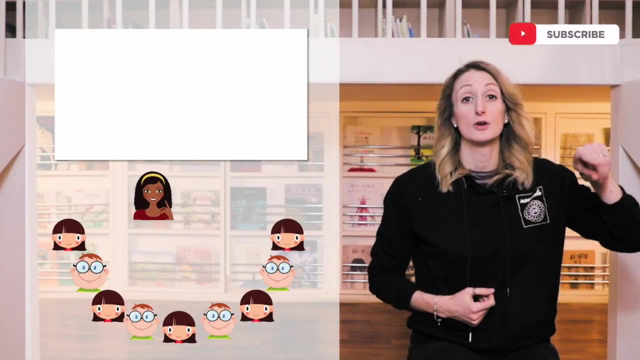 of the vocabulary you'd like to practice Now. in today's example, I'll be using fruits as a subject. However, you can adjust this game to suit any subject that you might be teaching. Start by positioning the class in a semicircle, with you, the teacher in the middle. 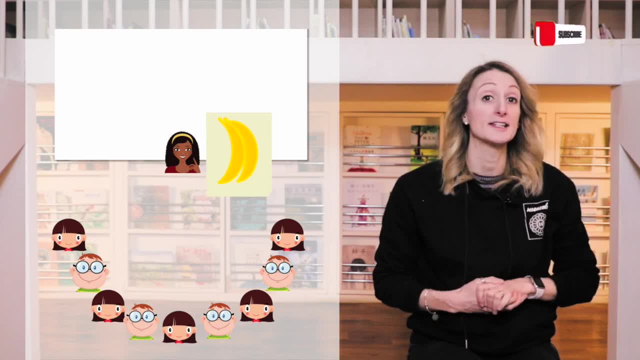 Next, you're going to introduce those flashcards one by one, using chance and TPR, as you do Now. if you're not sure how to use chance and TPR in your classroom, then make sure you check out my video on TPR, linked below. 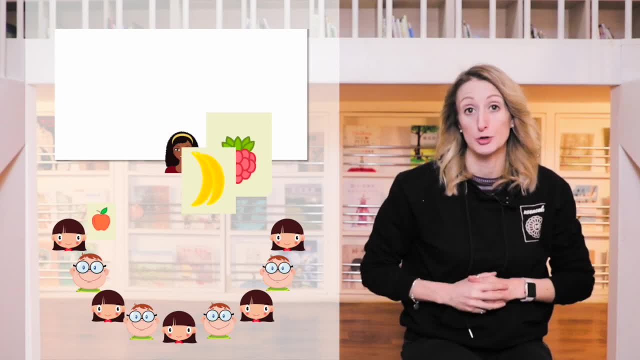 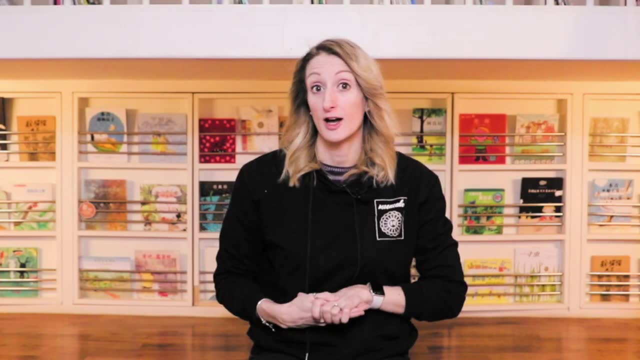 Next, you're going to take those cards, Give them a shuffle and hand them out to students. Every student should have one flashcard. Now, as you're doing this, you can add in some extra language points by having students ask for the card. 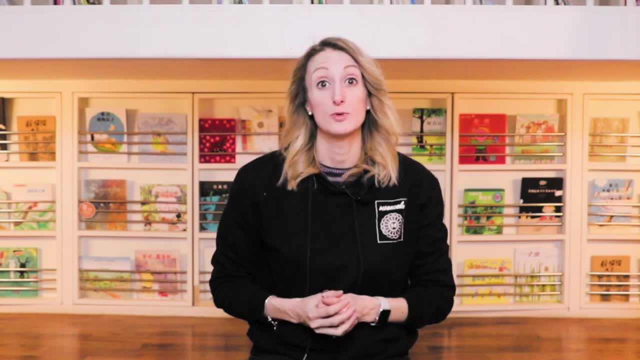 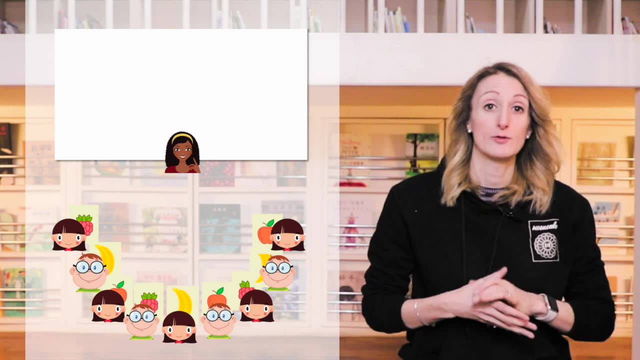 For example, may I have a card please? The whole class as a group can then ask the student receiving the card: what card do you have? And they can then reply saying: I have bananas. Once everyone has a flashcard, you're going to ask the whole class to stand up and listen very carefully. 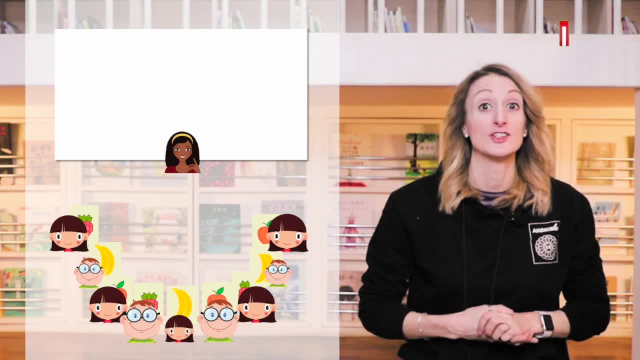 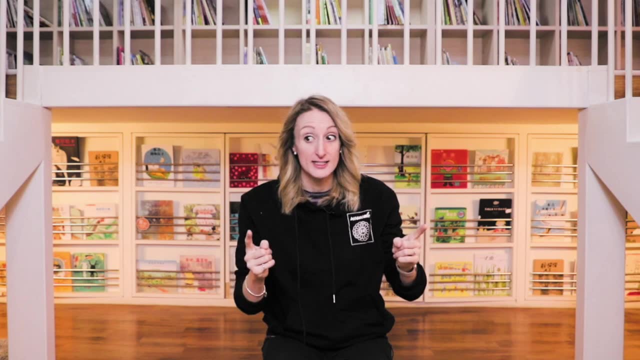 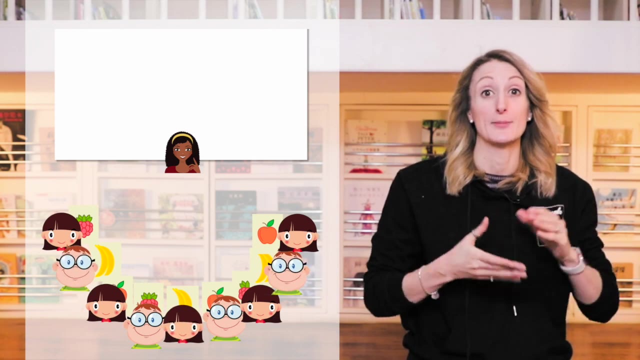 Choose one fruit and ask them to squat down as the whole class chants together: Banana squat, banana squat. think fast, think fast. apple squat. As soon as you change the name of the fruit to apple's squat, all those bananas need to stand back up and those apples need to squat down. 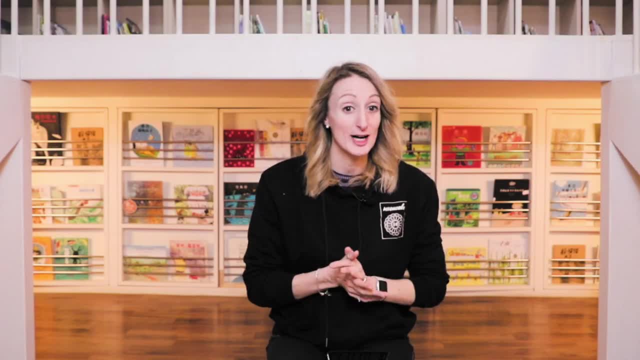 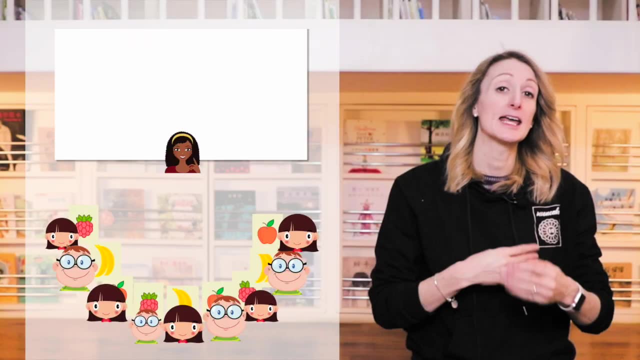 Once again, the whole class are going to chant together: Apple squat, apple squat, think fast, think fast. strawberry squat. Keep going again and again until all the vocabulary has been sufficiently drilled. Now to make this game even more fun. 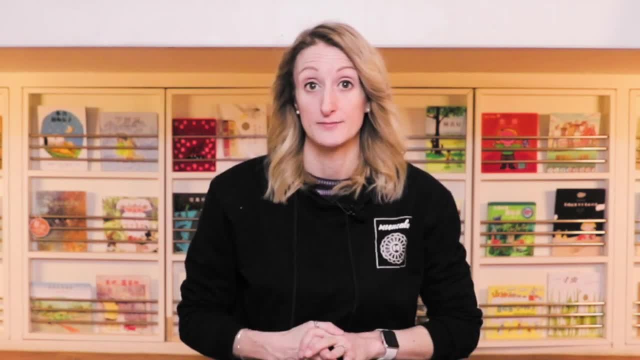 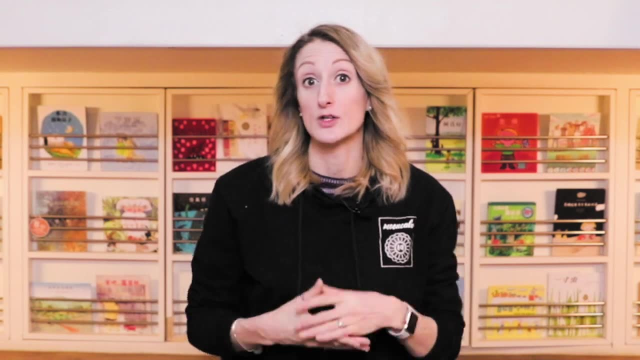 you can add in some competition by eliminating the slowest fruit. This way, you keep students' attention as they wait with anticipation to see if their card will be picked. Keep going again and again until there's only one fruit left. who is crowned the winner? 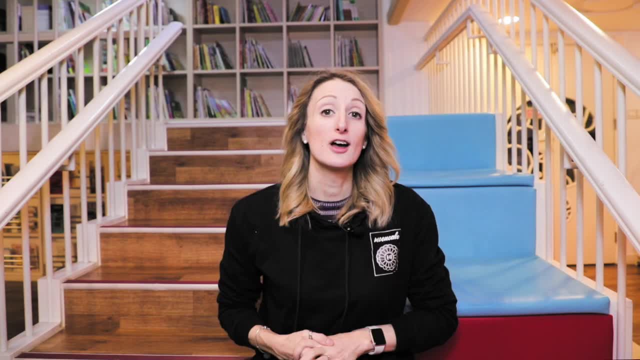 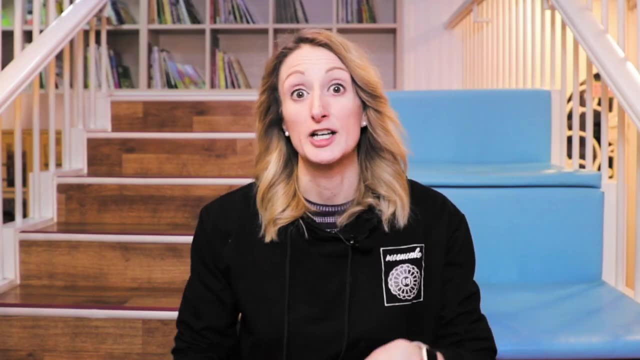 Now, if your class are a little, let's say, energetic, then you can calm things down by changing the actions in the game. So instead of squatting, you might have students put their hands up. It's always a good idea if you've done a high energy action. 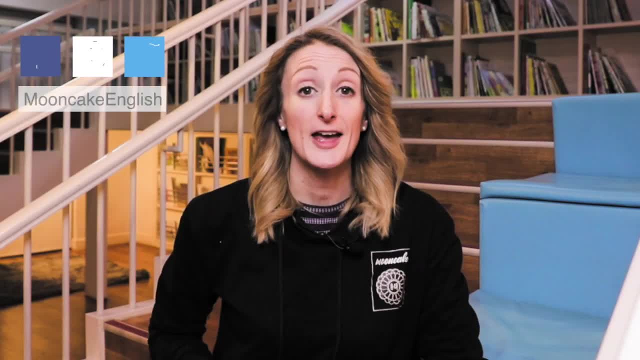 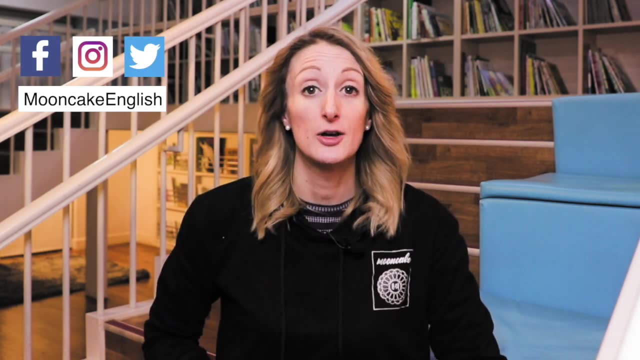 to then calm things down before moving on to another game. So they have There you have it: a fun and engaging way to practice new vocabulary. If you like this video, let me know by commenting the word helpful in the comments below and by sharing with your fellow teachers.